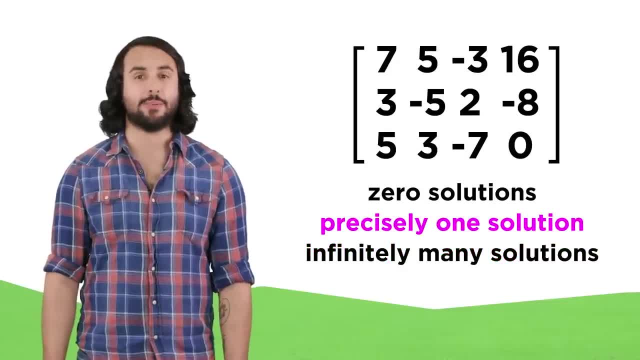 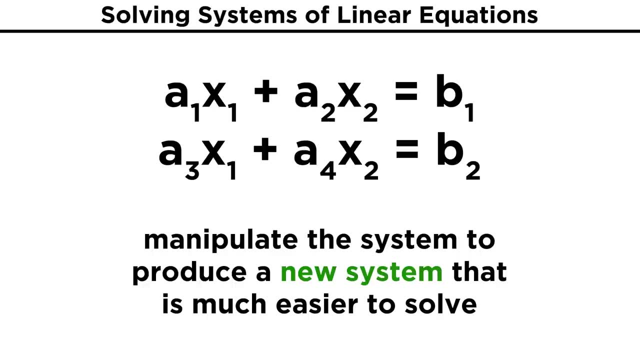 there is one solution. we want to find precisely what it is. What are some techniques that we can use to do this? The main strategy that we will use involves manipulating the system to produce a new system of equations with the same solution as the original one, but is much easier to solve. 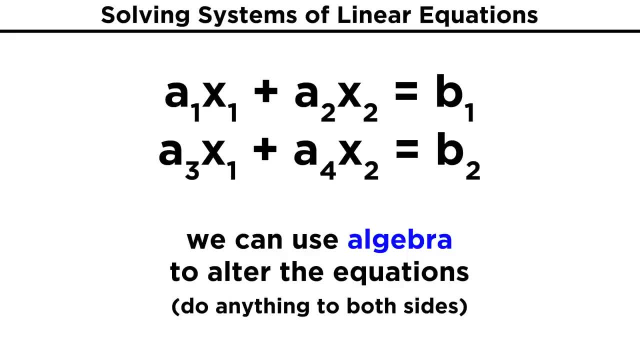 How can we do this? Actually, this is still the same concept that we learned in algebra: We can manipulate the equations in a system in any way we want. that is algebraically valid, meaning we can do anything we want to an equation, as long as we do it to. 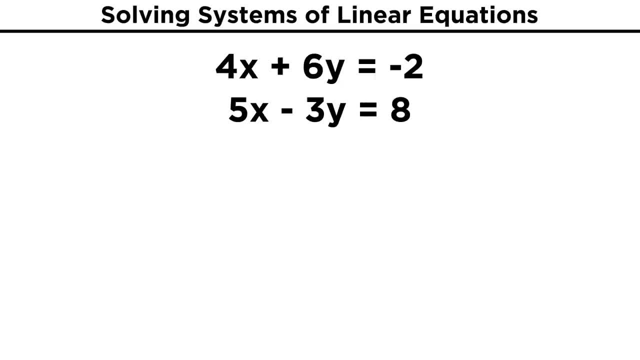 both sides of the equation. Say we have the following system of two linear equations: four x plus six, y equals negative two, and five x minus three, y equals eight. Let's go ahead and generate the corresponding augmented matrix, which will be two by three. 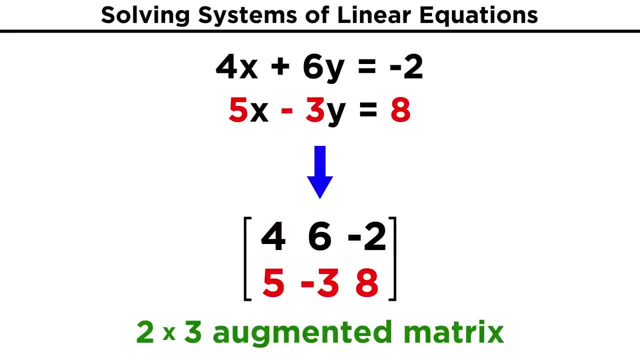 with four, six and negative two in the first row and five negative three, eight in the second row. One option available to us is to take any equation and multiply or divide the two linear equations by some number. How about we take the first equation and divide everything by two? 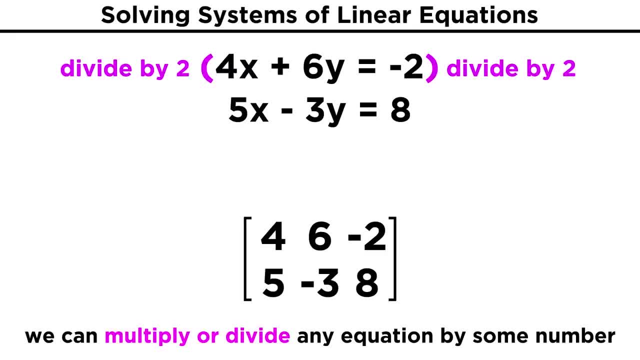 This shouldn't change the equation or the system, because everything will be in the same proportion. We can also just do this to each term in the first row of our matrix, but just for clarity, let's do both of these things so that we have equations to look at while we do matrix. 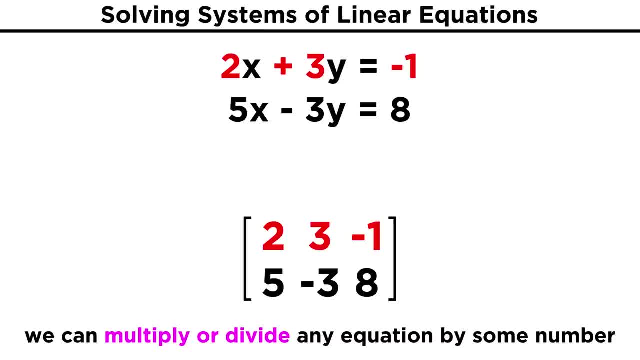 operations. Dividing through, we get two x plus three y equals negative one and we alter our matrix accordingly. We can multiply or divide any equation in this manner, or the corresponding row by any number we want, except for zero. The reason we divided by two is simple, because now we can use another technique. 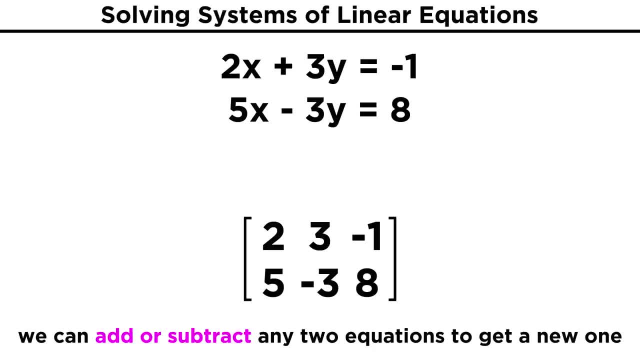 We can take any two equations in the system and add or subtract them to produce another valid equation that will be part of the system. This is another technique we learned in algebra. Now with the matrix, we want to retain our matrix, We want to retain the dimensions of the matrix. so let's say we decide that we want to add. 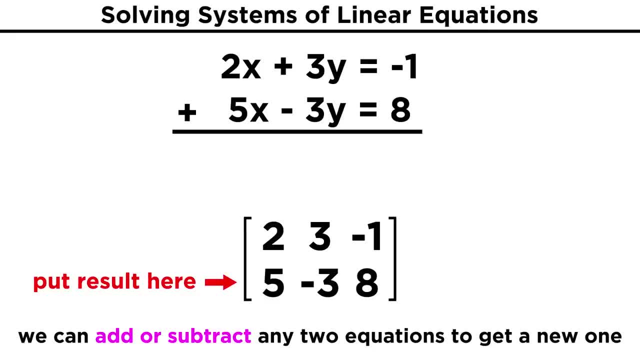 the two rows together. Let's do so and replace the second row with our result. We can achieve this by adding the values in the first row to the values in the second row. below To five: we add two and get seven. To negative three, we add three and get zero. 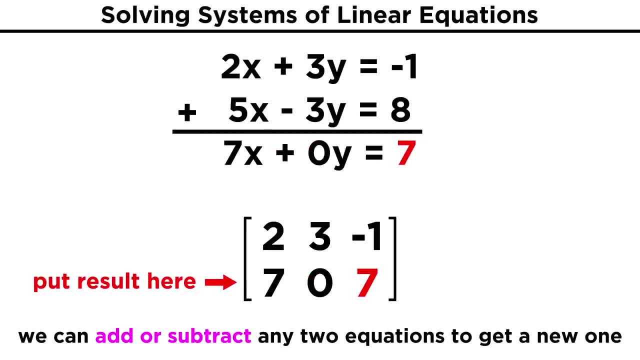 To eight, we add negative one and get seven. So, to summarize, We can add or subtract any two rows to generate a new row without affecting the solution to the system, Combining this with the previous technique where we could multiply or divide any row. 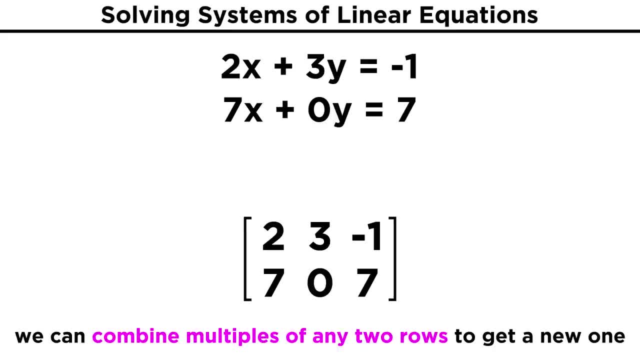 by some number. we can actually add or subtract any multiple of any row to any multiple of any other row to get a new row, or even simply swap two rows without changing any of the values, all without affecting the solution to the system. Okay. 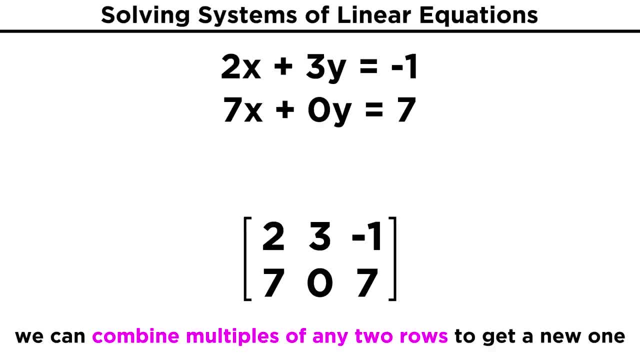 opens up a lot of possibilities for what to do with a system of equations. Now take a look at what we are left with in the second row: seven zero seven. This is the same as the equation: seven X plus zero Y equals seven. 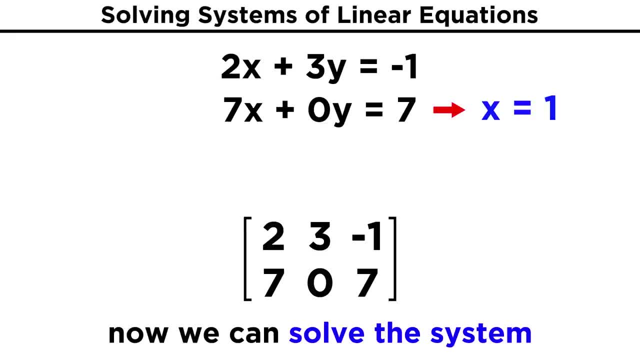 This is trivial to solve: X equals one. Plugging that into any other equation, we end up with negative one for Y and we have solved the system. So, as we can see, the key is getting rows with zeros in them. If we took this row and divided by seven, we would get one zero one, and then we don't. 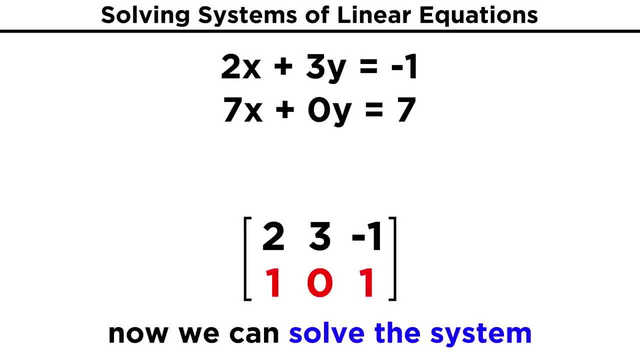 even have to use any equations. The matrix spits out the answer. So the goal for any linear system is to write out the augmented matrix and do elementary row operations until each row has a one in one of the columns and zeros in the rest. 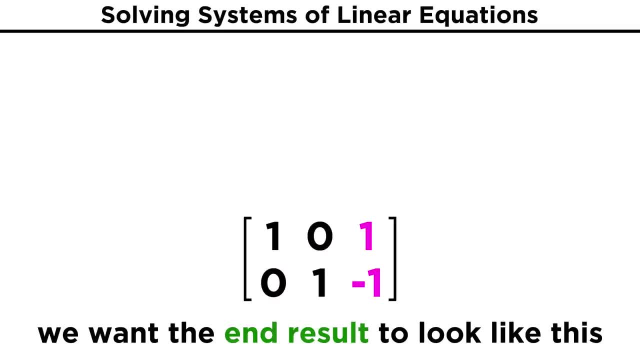 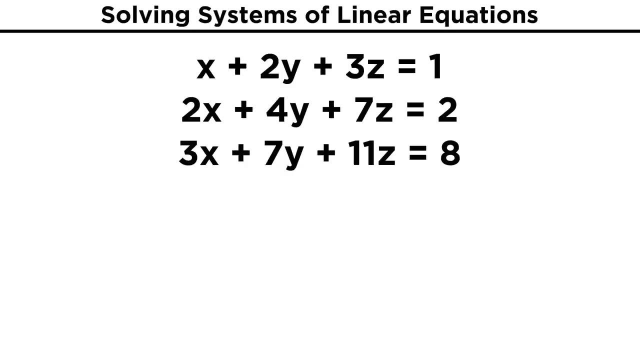 except for the rightmost column, which will give us the value for the variable that corresponds to the position where the one is located. When we perform this on a matrix alone, this technique is called Gauss-Jordan elimination. Let's go through one full example together. 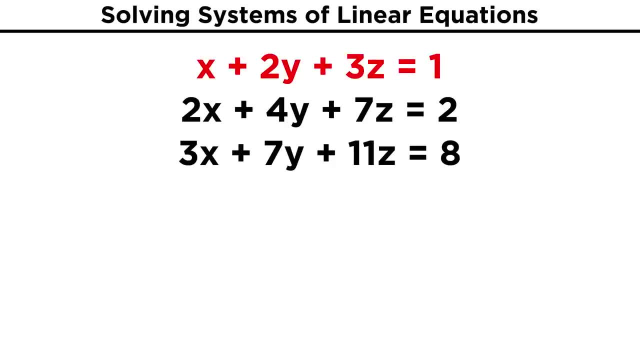 Take the following equations: X plus two, Y plus three, Z equals one. two, X plus four, Y plus seven, Z equals two, and three, X plus seven, Y plus eleven, Z equals eight. So the answer is two. Let's go ahead and construct our augmented matrix, which will be a three by four matrix. 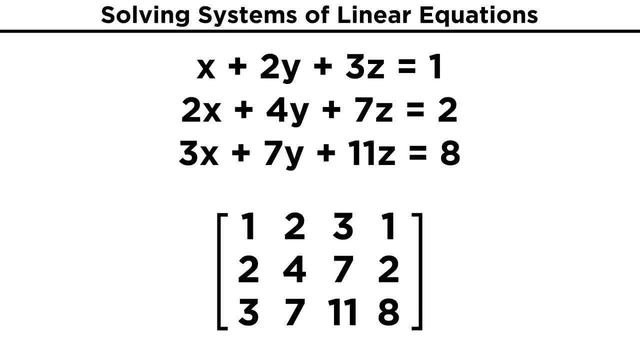 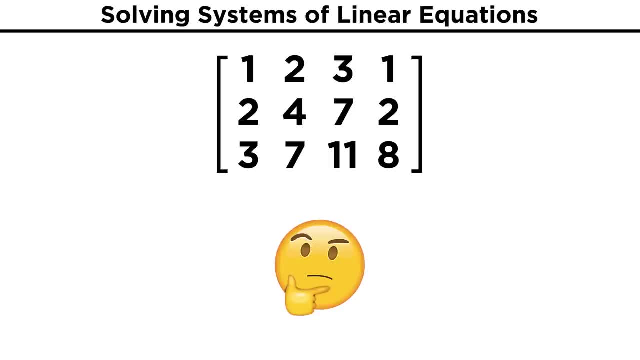 since we have three equations and three unknowns. Now what elementary row operations jump out at us? There are plenty of ways we could do this. One thing we could notice is that the coefficients in the first column are one, two and three. 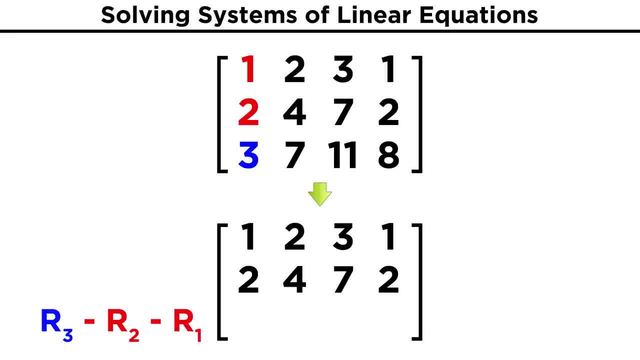 What if we subtract both the first and second row from the first column? So what happens? We subtract both the first and second row from the third row to get a new third row. Three minus two minus one is zero. Seven minus four minus two is one. 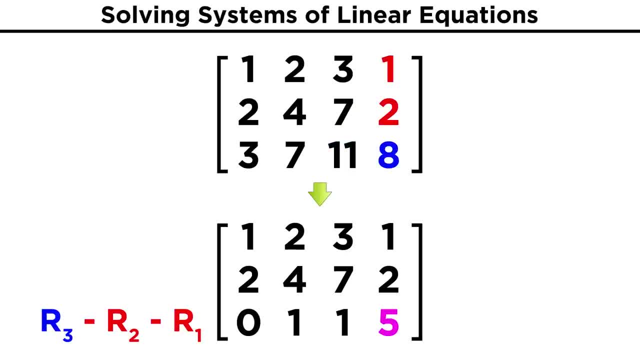 Eleven minus seven minus three is one, And eight minus two minus one is five. Getting a zero is always productive, so that was a good start. What next? Let's say we notice that the first two coefficients in the first row are precisely half the corresponding. 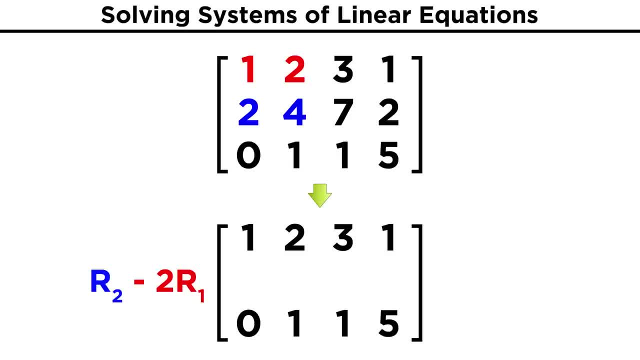 zero. So what we can do is subtract twice the first row from the second row to get a new second row. So two minus twice one is two minus two or zero. Four minus twice two is four minus four or zero. Seven minus twice three is seven minus six or one. 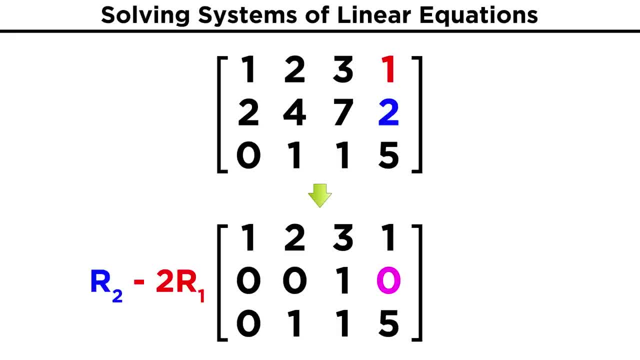 And two minus twice. one is two minus two or zero. That was a very productive move, because we have just solved for two. I'll see you next time. one of the variables, z, must be equal to zero. Now we are in great shape to solve for x and y. 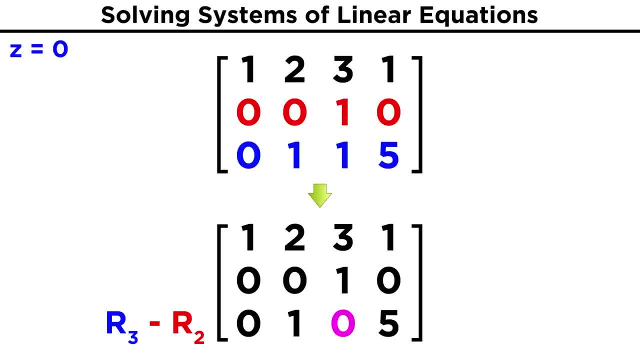 Let's subtract the second row from the third row to get a new third row, because that will get rid of this one in the third position. And now we have zero one, zero five. That means y must be equal to five. 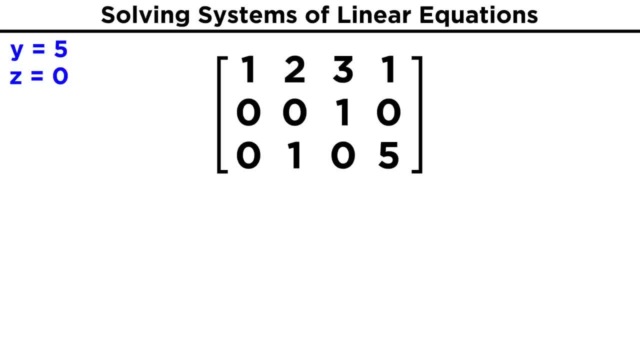 And now it's easy to finish things off because we have two variables isolated: The first row minus twice the third will give us one zero three negative nine, And then from that we can subtract three times the second row to get one zero, zero, negative. 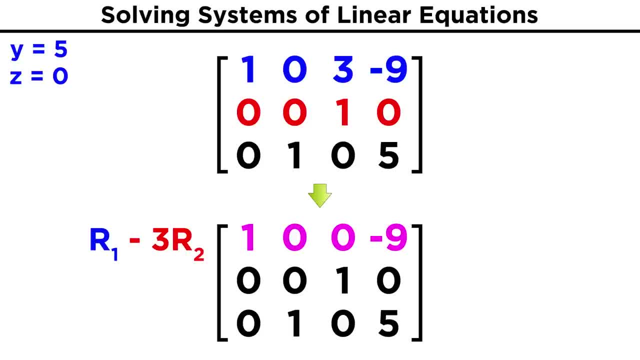 nine. Just for the sake of aesthetic, let's swap the position of the second and third rows so that we have the ones along the third row, And that leaves us with our solution spelled out for us, nice and easy. X is negative nine, y is five and z is zero. 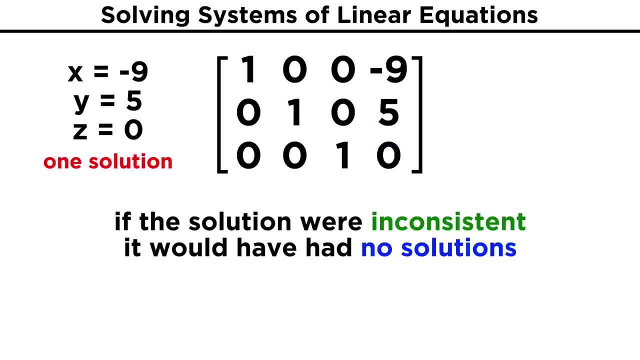 Once again, we could have ended up with no solutions if the system was inconsistent, or we also could have ended up with infinitely many solutions, but in this case we got just one. There is a way to tell how many solutions there are once Gauss-Jordan elimination is. 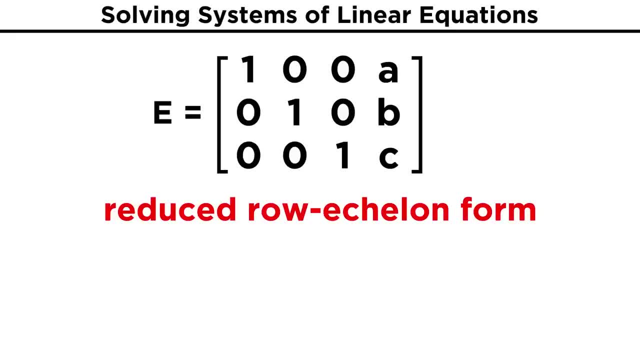 complete. It will be the case once the matrix is in reduced row echelon form, which can be abbreviated this way: A matrix is in reduced row echelon form when any row with non-zero entries has a one as its first entry. This is called a leading one. 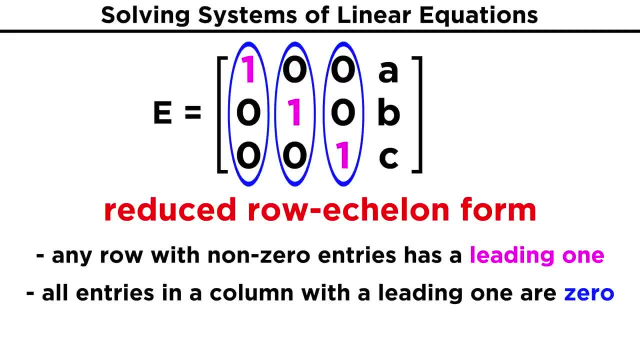 Wherever there is a leading one, all the other entries in that column are zero, and for any row with a leading one, there is a leading one in the first column, and for any row with a leading one, there is a leading one in the second column. 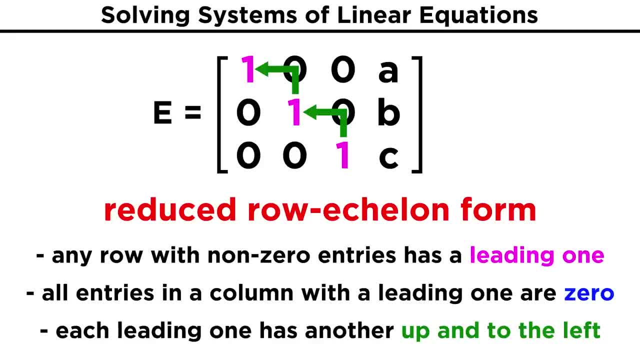 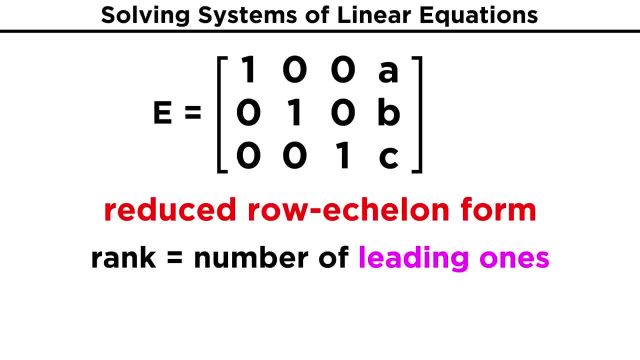 However, there is a leading one in the row above that is, further to the left. Once we have a matrix in this form, Gauss-Jordan elimination is complete and we can look at the rank of this matrix. The rank is the number of leading ones. 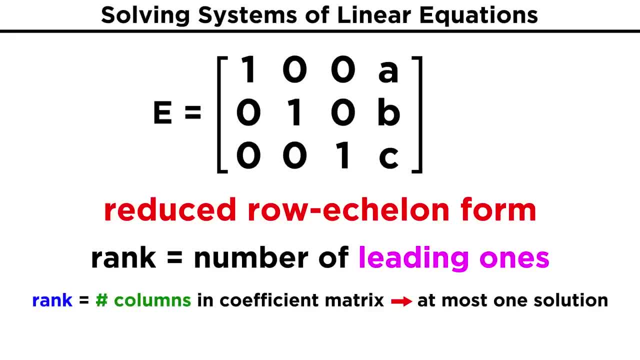 If the rank is equal to the number of columns in the coefficient matrix, the system has at most one solution, meaning this will typically result in a unique solution. If the rank is less than the number of columns, it's not one. less than the number of columns in the coefficient matrix, the system has either infinitely many,